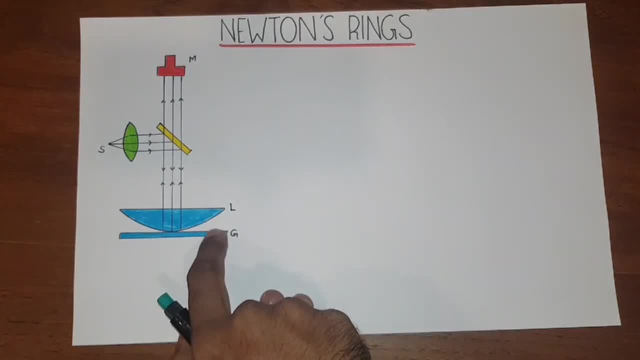 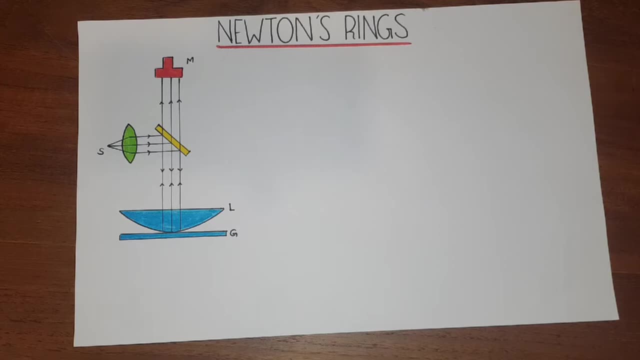 of this film and also from the bottom part of this film which will interfere to create a pattern. So we will be using the cosine law where we can manipulate the thickness part to find the interference pattern conditions. So here at the center, the glass plate and the lens. 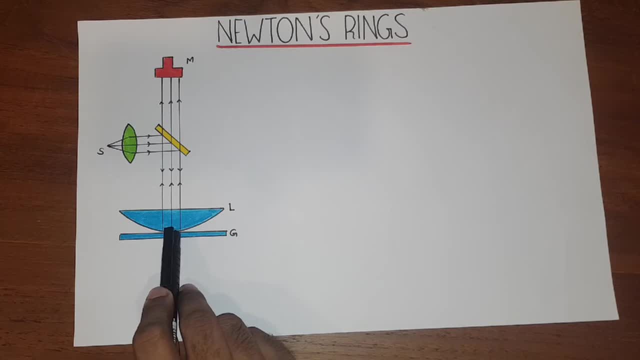 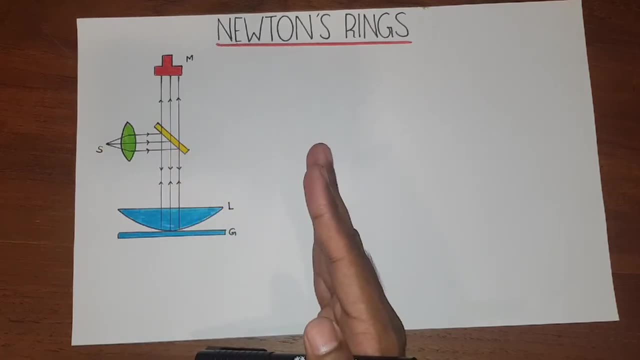 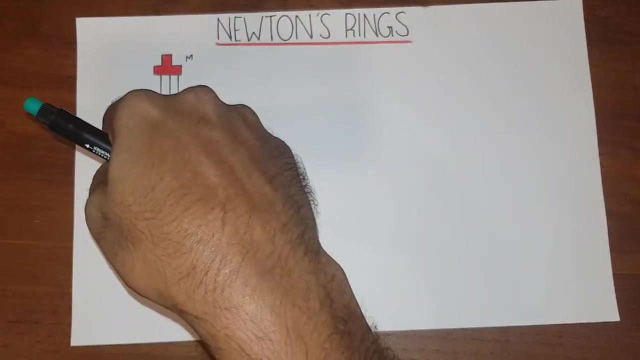 is touching. So there is no thin film, the presence of thin film at this central point. and as we go outwards, the thickness of the thin film goes gradually increasing. But this is in a circular way. if you just imagine this in three-dimension. if you look from the top part, the same thickness. 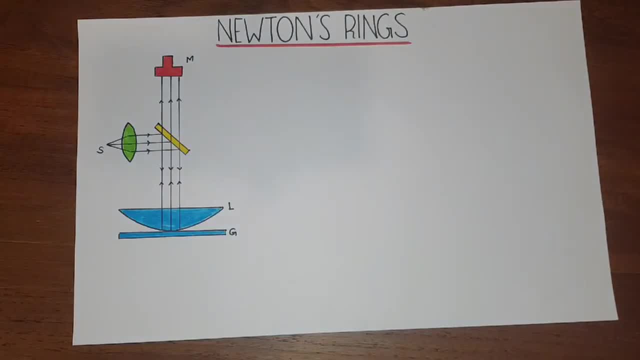 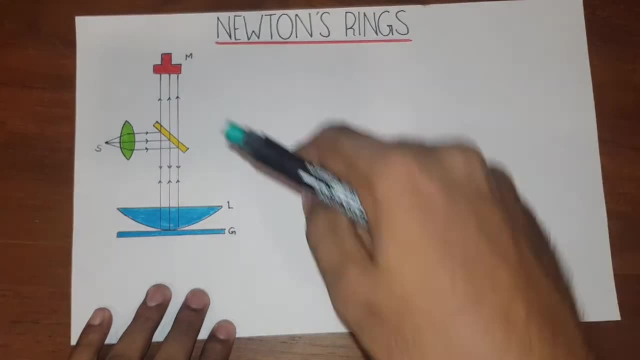 part will be in the form of a circular shell, Because if I consider the end, most part, the locus of all, the end point will be a circle. Similarly, if I concentrate point somewhere in-between, 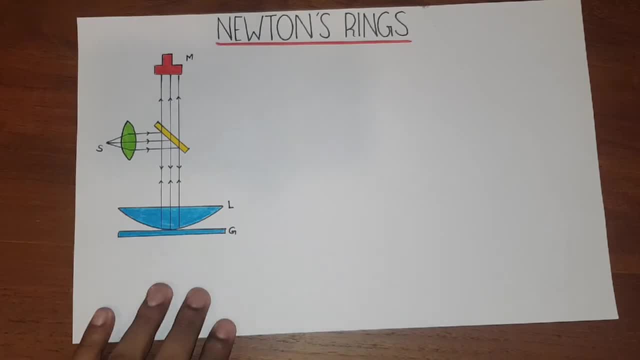 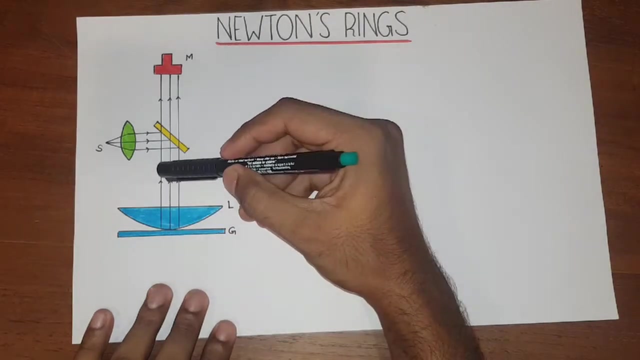 locus of all the points having the same thickness will be a circle. now let's start from the beginning, like from the central part. if we look at the centre, there is no film, but even there light is getting reflected from the bottom part and the top part and between these. 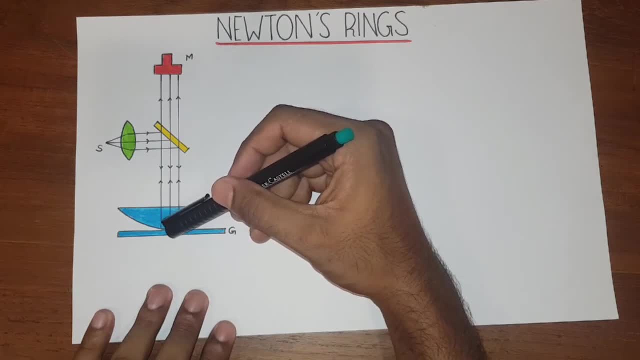 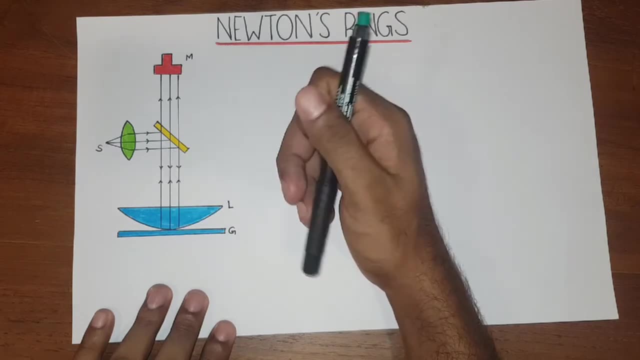 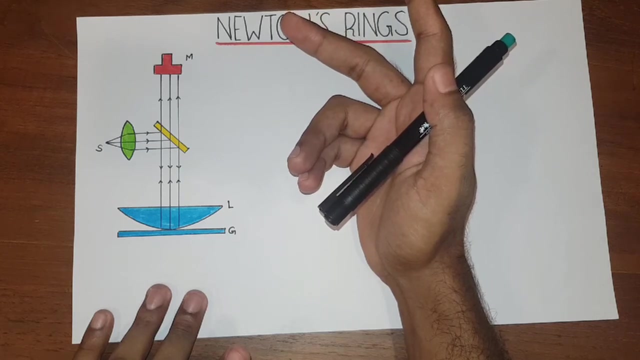 two rays there will be a path difference of lambda by 2 or a phase shift of 18 degree. so these two rays will be interfering destructively, which we already know, that any two rays which have a path difference of lambda by 2 will always interfere destructively. so always at 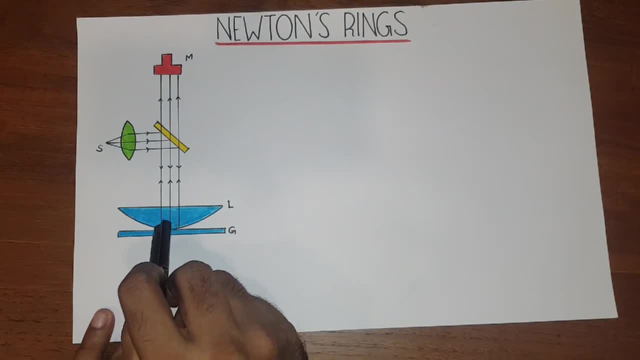 the centre or the central band or the central fringe. Newton's ring will be a dark fringe which is always in1. sohow do we know that the iris's謝 힘들by is Being Disturbed? That has changed your sleep thread последarly. as you change it, your sleep thread is also. 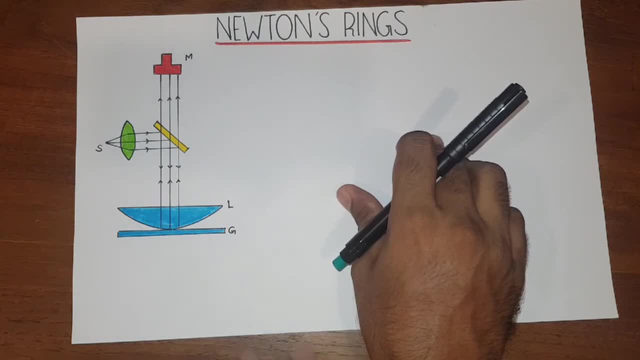 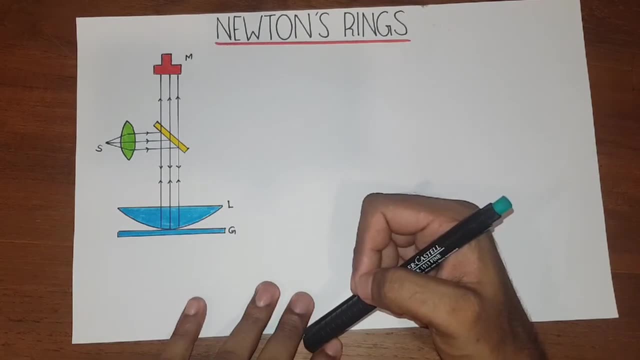 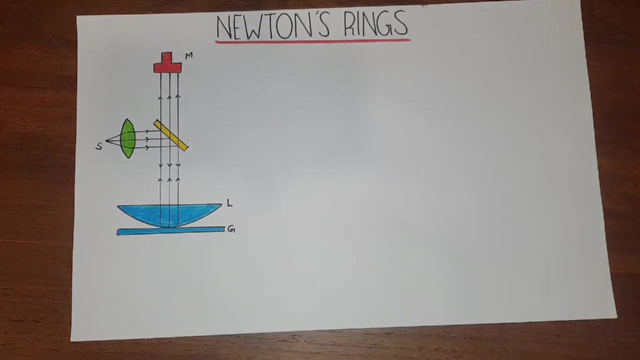 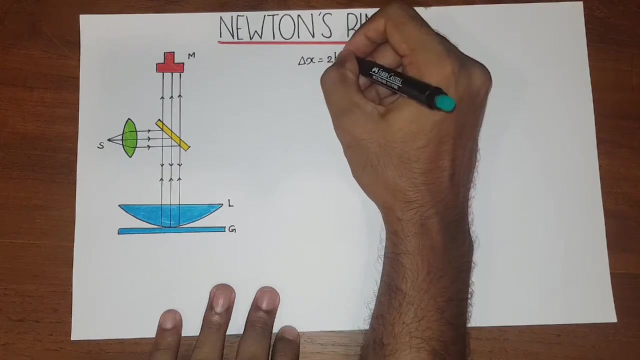 because the rays from this part will be interfering destructively And as we go outwards towards this film. how can we know how the rays are interfering? We have to measure the path difference and the path difference formula we already know from the cosine law, that is: delta x equal to 2 mu t cos r. 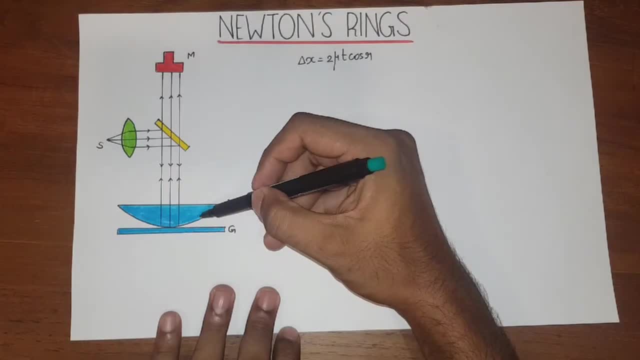 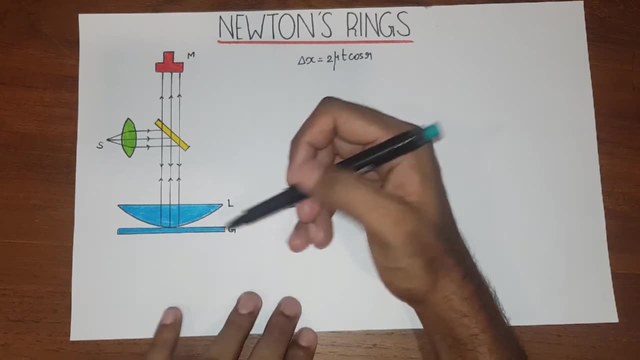 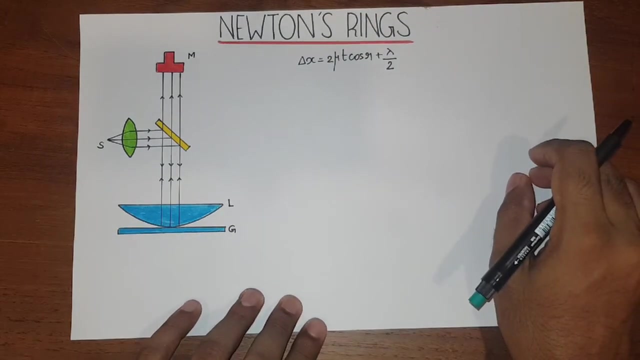 And just like the air wedge case, there is a ray getting reflected from the top part suffers no phase change. but there is another ray which is getting reflected from the bottom part which will suffer a path change of lambda by 2, which has to be taken into account. 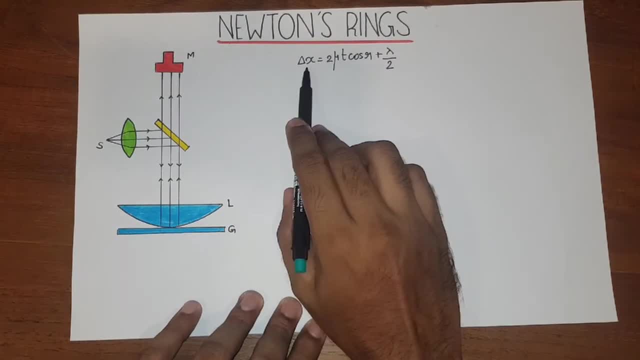 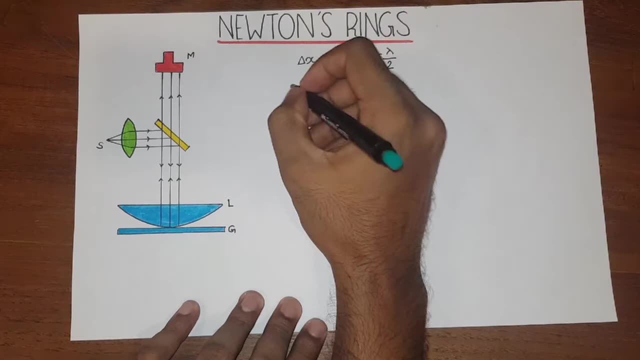 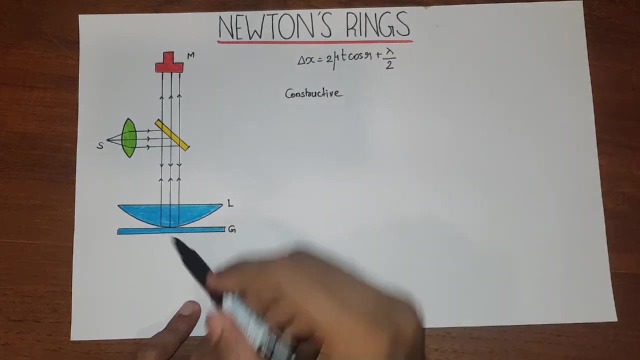 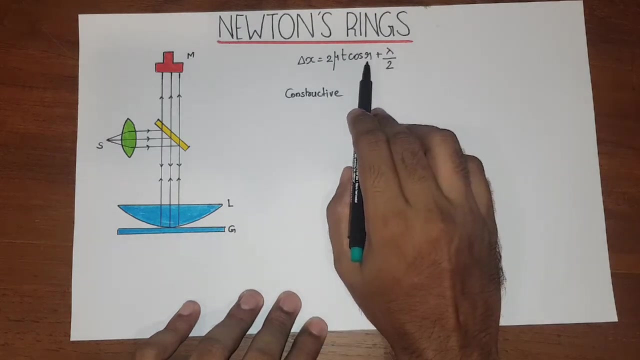 Now what we have to do? Now, what we have to do is Substitute the value of delta x for constructive and destructive patterns. So let us now first consider the constructivities, or constructive interference. So here also, since it is a normal incidence, phenomenon r can be limited to 0.. 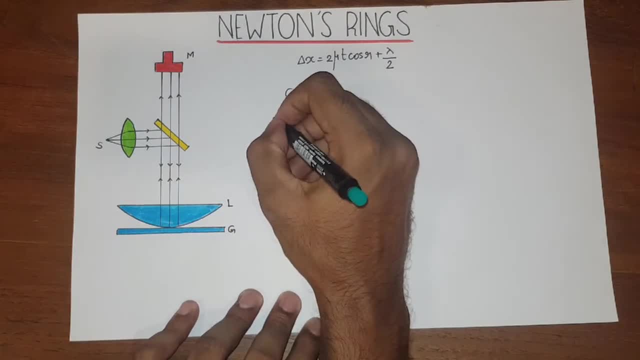 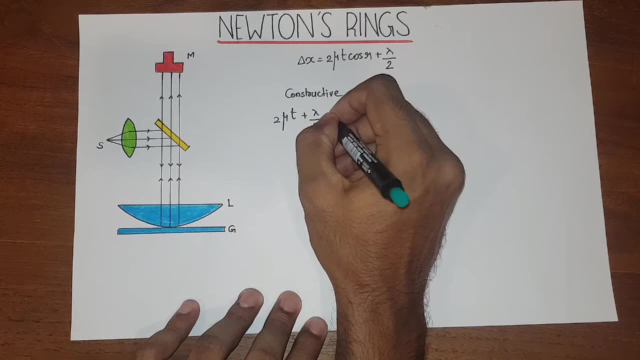 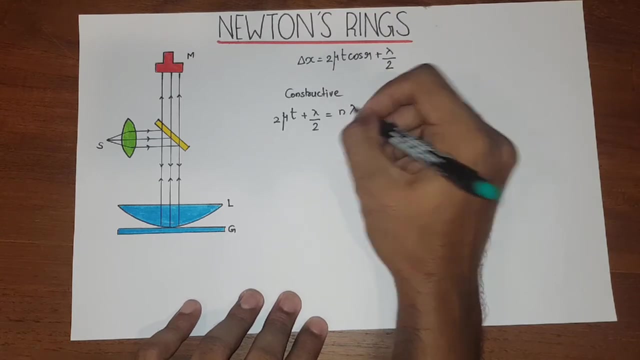 So cos r value will be 1.. So this equation can be written as: 2 mu t cos r will be 1 plus lambda by 2 will be equal to what will be the value of delta x for constructive interference. For constructive interference this will be n lambda. 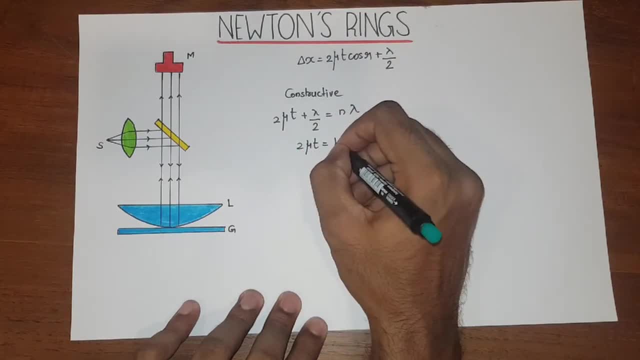 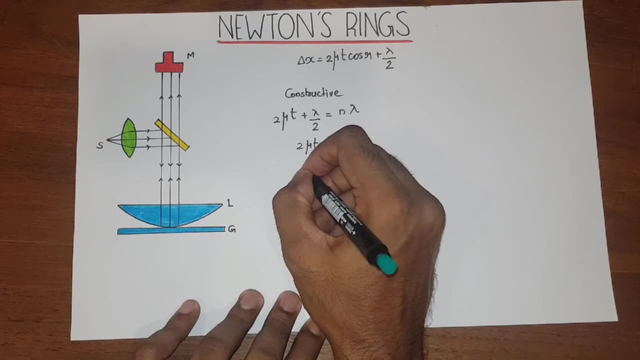 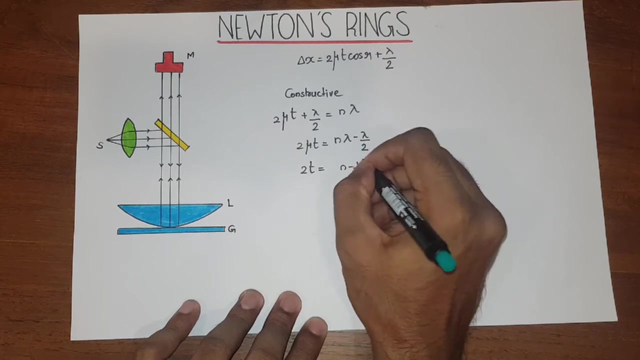 And 2 mu t will be n lambda minus lambda by 2, which is n minus half into lambda. So I am retaining this 2t over here and bringing all of the things to the right hand side. that is n minus half lambda on the right hand side and I have to bring this mu to this side. 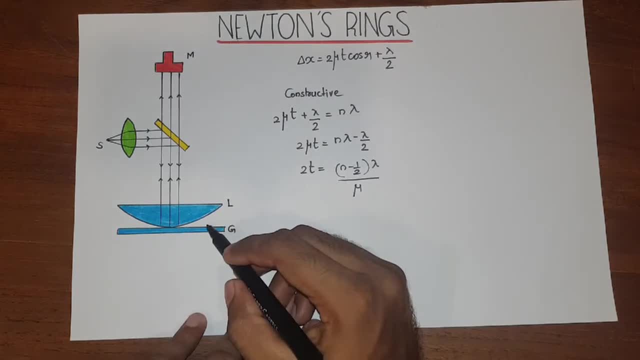 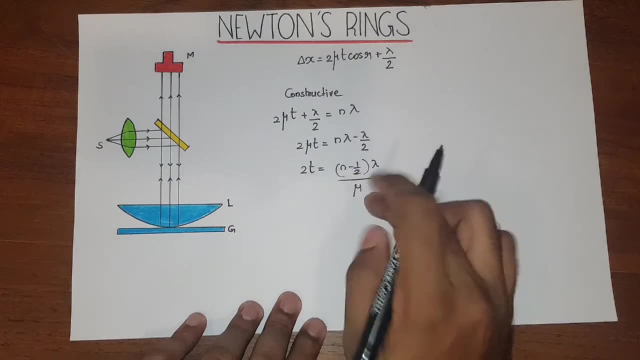 So retaining this mu is your choice, because if this space is filled with air, the refractive index will be 1, so you can omit this part. but that is your choice, because if it is not air and if it is some other liquid, this mu value will become handy. 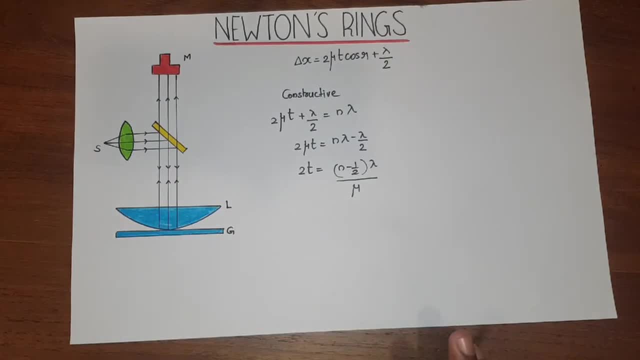 So I am retaining this 2t. Why did I do this earlier in the air wedge case? what we did was we linked the thickness to the x value. So instead of using thickness in the equation in the case of air wedge, we substituted the x value, that is, the distance from one end of the glass plate to the point where we are. 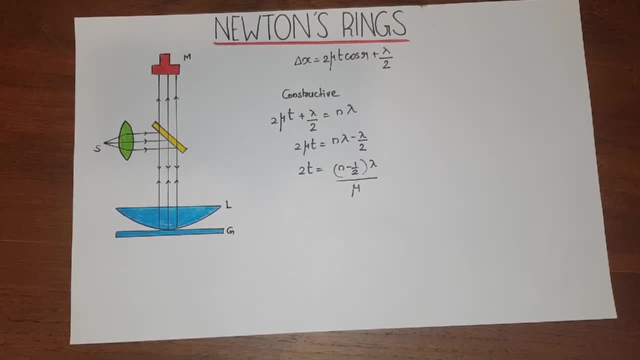 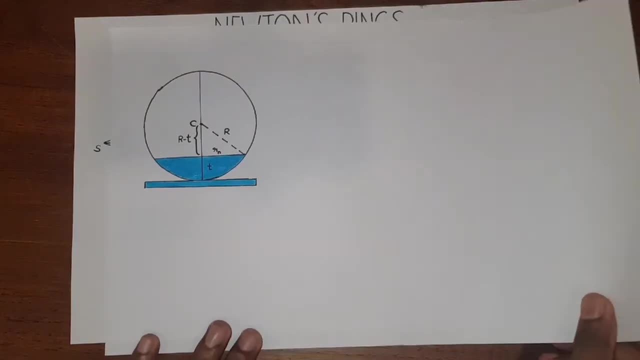 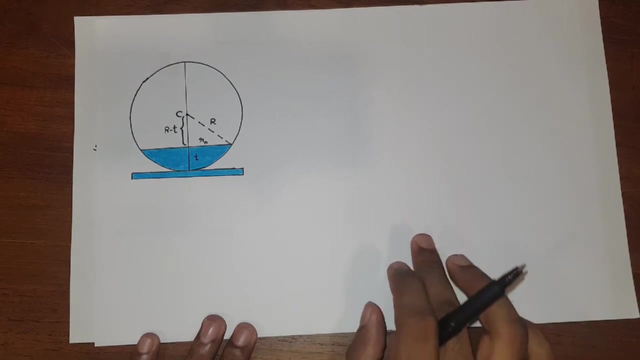 observing the fringe, so that that value can be directly measured by using the travelling microscope. a similar thing has to be done here, but here, instead of measuring the position, here we are going to measure the radius. or I can say that instead of using the thickness now I am going to convert the thickness into a radius format so that it is measurable with. 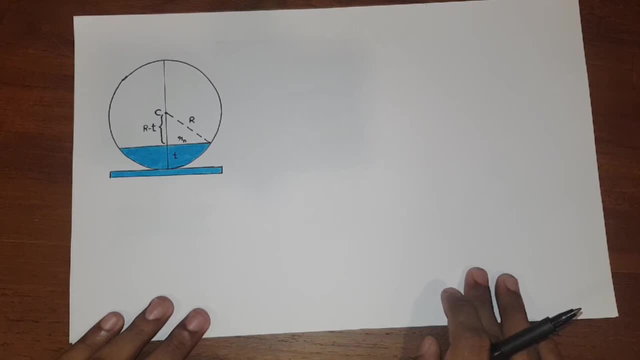 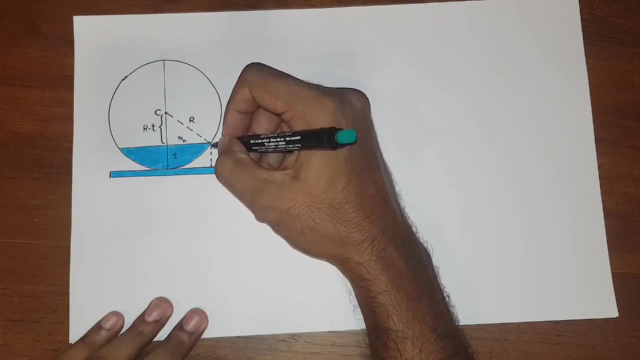 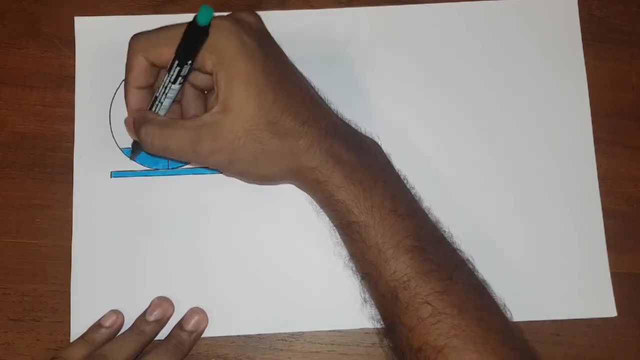 the help of a travelling microscope. So I am considering a random equation. So I am considering a random equation, So I am considering a random point over here, or I am considering the part of the film which has this thickness t, and the same t is available here and from this I have completed the circle. 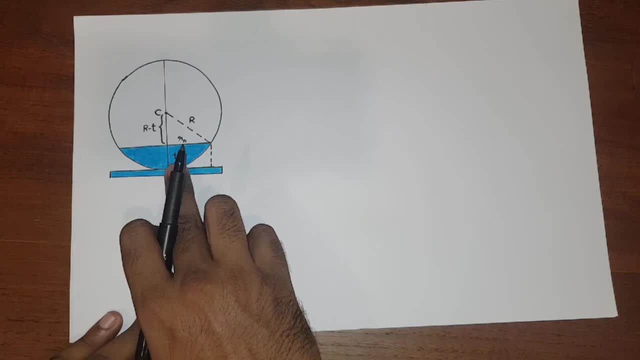 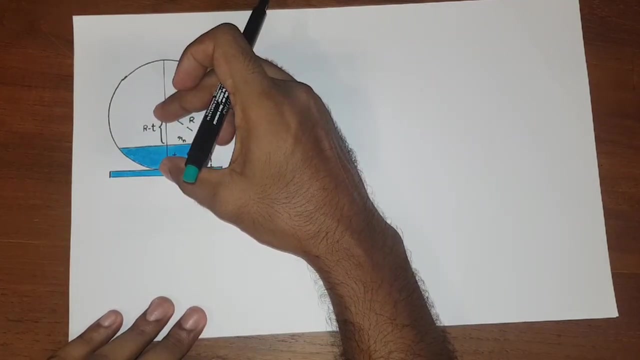 of which the length is a part- let us say our elementary school knowledge that every length is a part of a circle, and then this length will be the radius of curvature of this length. So this part will be the radius, and this part will also be the radius, and this is the thickness part. and if you subtract this, 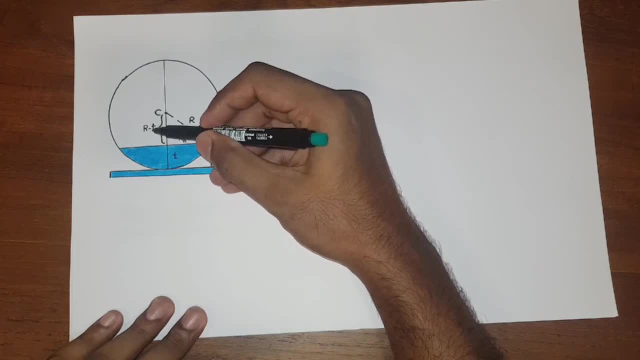 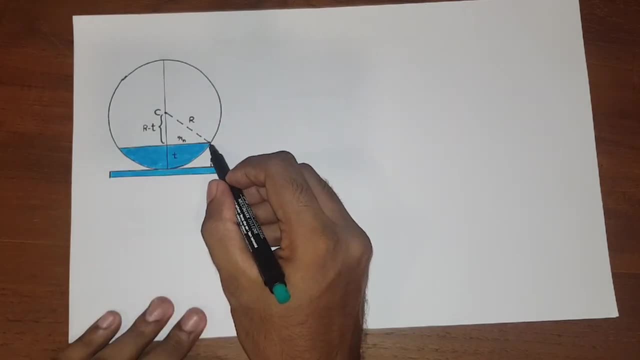 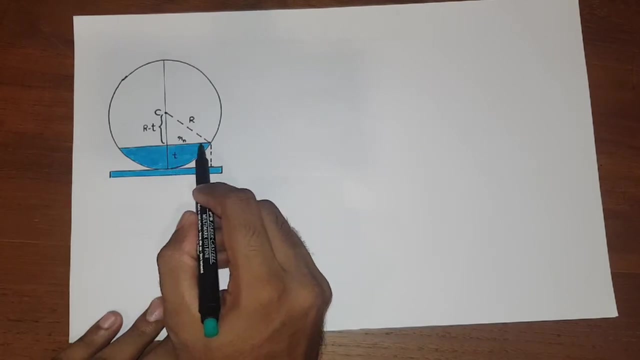 thickness from the whole radius. this distance will be radius minus the thickness, and this distance will be the radius of the ring which you will be observing at this point, Due to this part of the film. there will be a ring which will be formed and this distance will be the radius of 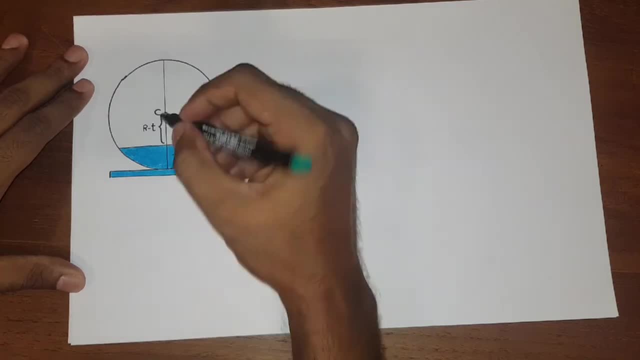 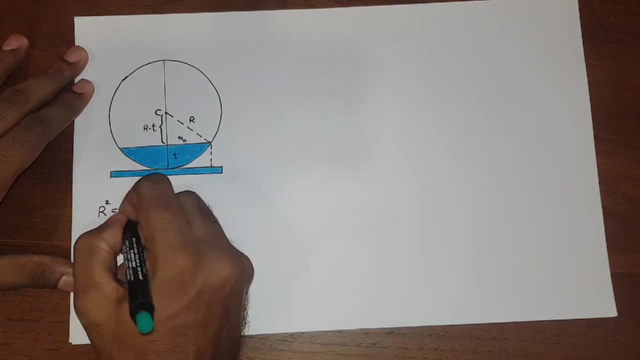 that particular ring. Now to this triangle. if you apply the Pythagoras theorem, you can write: I put you square equal to base square plus altitude square. On expanding this bracket value, you will get Rn square plus R square plus t square minus 2Rt. 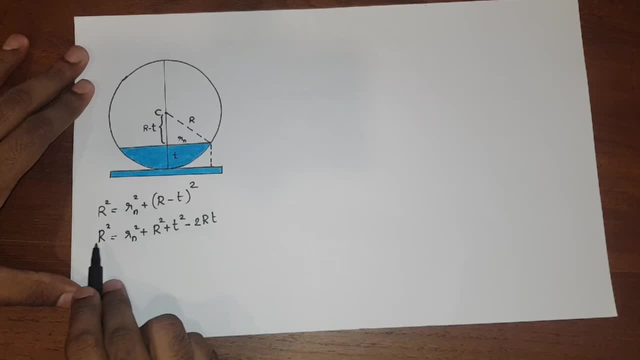 Here we have R square and this R square and this R square will cancel out This 2Rt and t square will come to the left hand side. So 2Rt minus t square will be Rn square. but when you consider these two terms, this is a very big term because usually the thickness will be very small. The 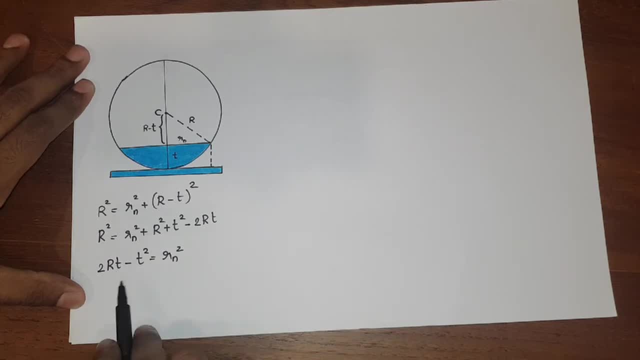 thickness of the film is usually very small, So t is small, So t square will be very, very small. So you are subtracting a very small value from a big value, So this can be neglected. This t square part can be neglected, So you can write it as 2Rt equal to Rn square. 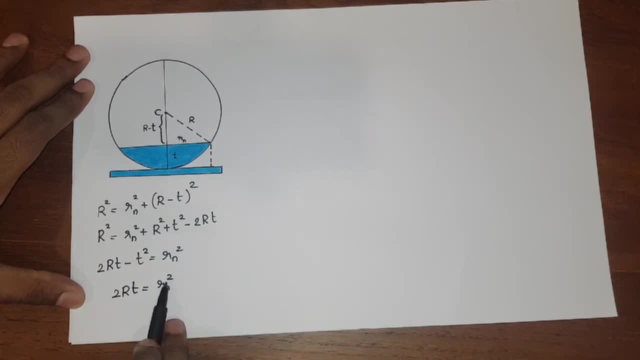 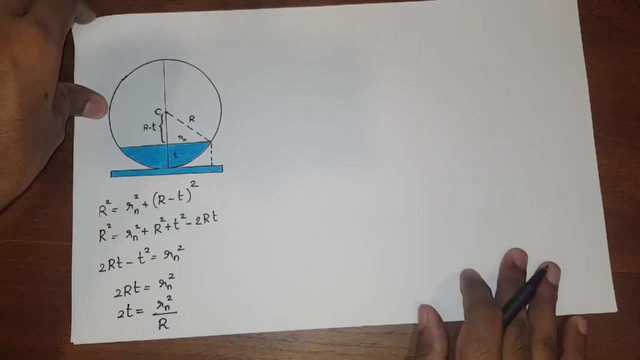 That is the radius of the nth ring. You have to square that term. You will get the term 2Rt, So you can retain the 2t. that is Rn square divided by the radius of curvature of the legs. So 2t is Rn square by R, and that is why I retain this 2t over here. So instead of considering the 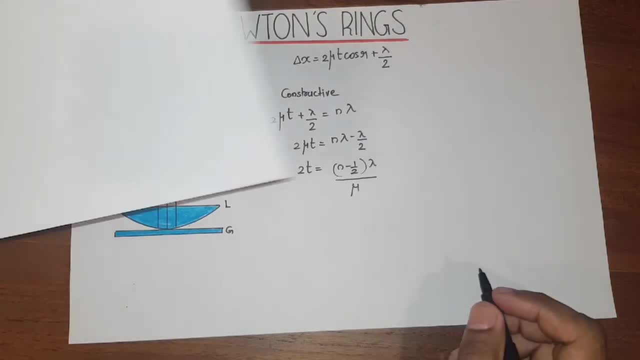 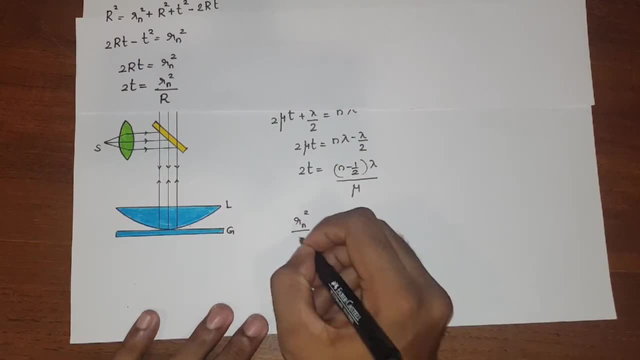 thickness. you can just substitute this value over here What is 2t. 2t is nothing but radius of the nth ring square divided by the radius of curvature of the lens, which is equal to. I am simplifying this, that is 2n minus 1 into lambda, the whole by. 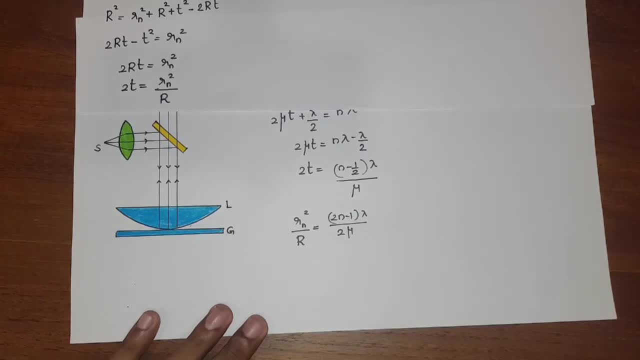 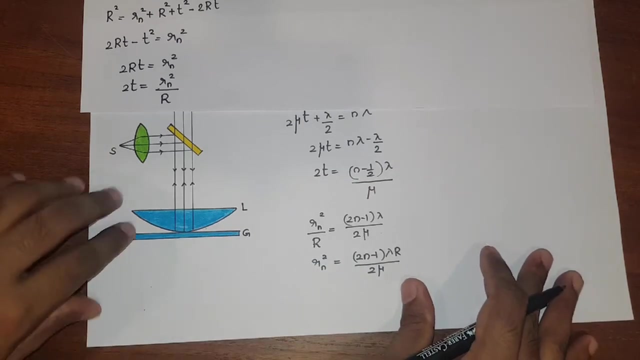 2 mu, And from this expression you can write: the radius of the nth ring square is equal to 2n minus 1 into lambda R divided by 2 mu, And from this you can directly write the equation for the diameter as well. Alright, I will do it step by step, I am just going to do it from here. 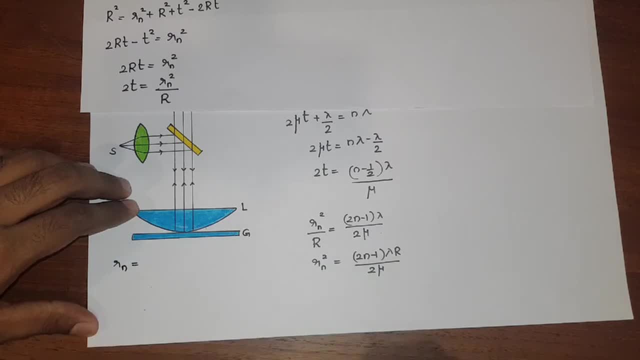 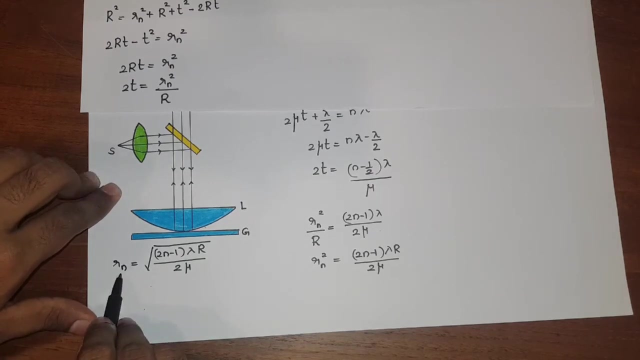 So I am just taking the square root. So I will get Rn, equal to square root of 2n minus 1, into lambda R divided by 2 mu. Remember that this mu can be omitted because if it is there, mu value will be 1.. I am now retaining it. That is your choice. So if we have the radius, then just multiply. 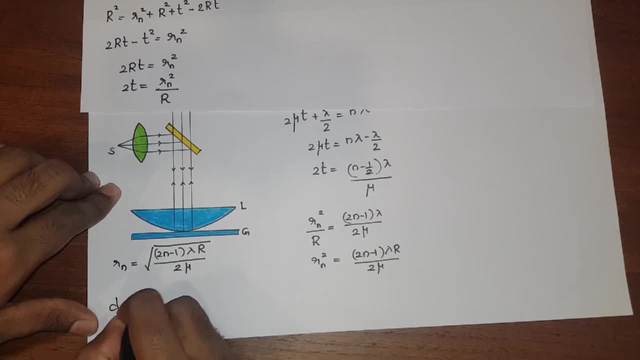 both sides by 2 you will get the value of diameter. So bn will be equal to multiplying this side by 2.. The 2 I am taking inside the square root. So I will get square root of 4 into this term So that 4 and 2 will cancel out. So 2 into 2n minus 1. 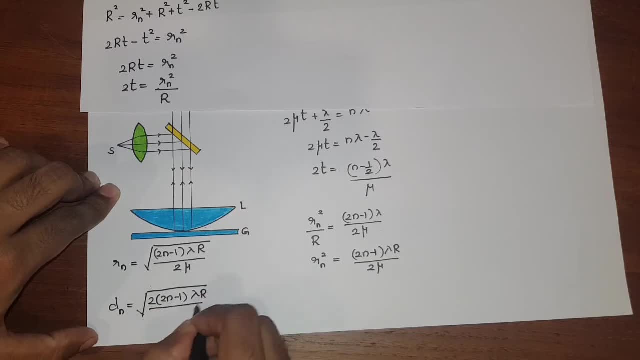 into lambda R divided by the whole thing is inside the square root. Or I can simply write it as: bn is equal to square root of 2 into n minus 1 into lambda r if mu value is equal to 1.. This is the expression for diameter. 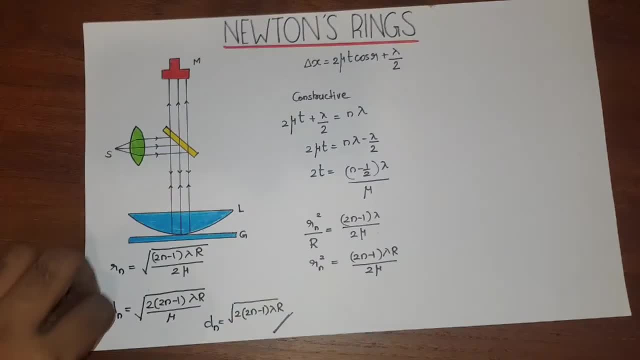 of the entry. And what condition did we apply? over here, We applied the condition for constructive interference, So at whatever. so, when you observe from the microscope, you will be seeing several rings, And whichever ring has this diameter or has this diameter which satisfies, 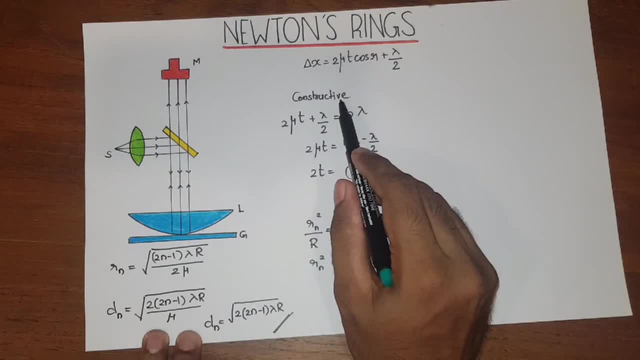 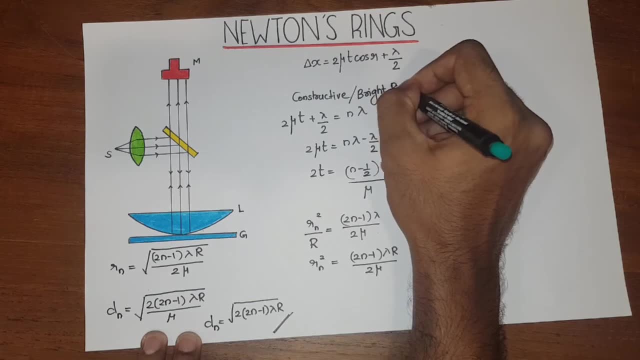 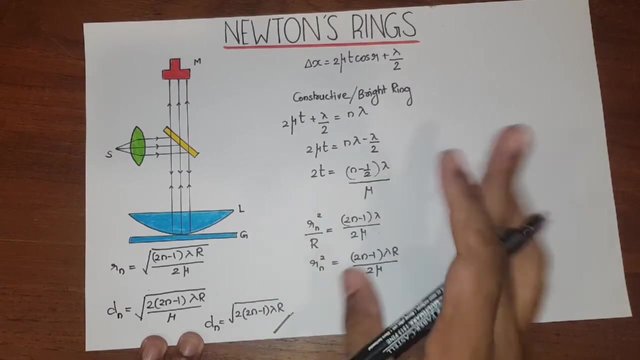 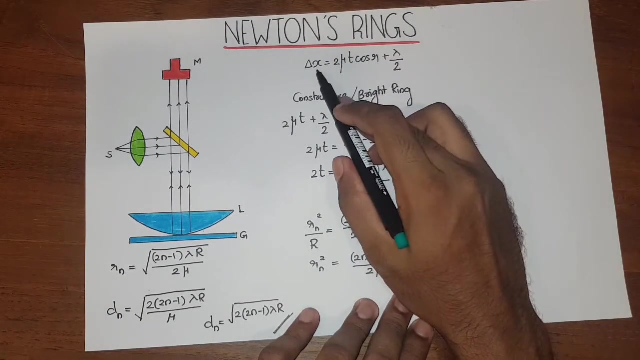 this condition: that ring will be a ring which is having constructive interference, or that will be a bright ring. So, whichever ring that satisfies this condition, it will be a bright ring. So what can we do next? So, instead of this, n lambda, so here delta. 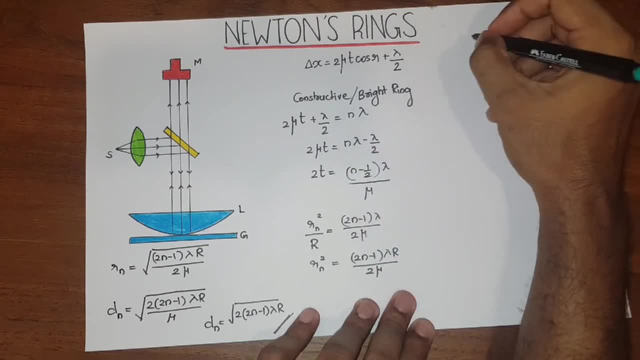 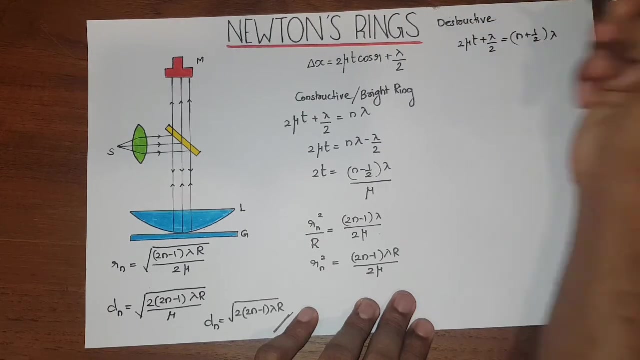 x we substitute as n lambda. So instead of n lambda. if I substitute 2 mu t plus lambda by 2 is equal to: instead of n lambda I am putting n plus half into lambda. What is that condition? That is the condition for destructive interference. Then 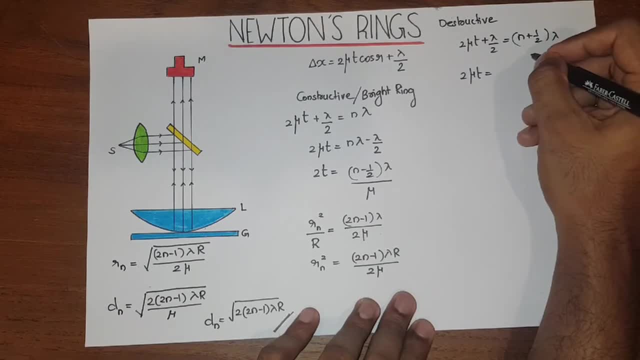 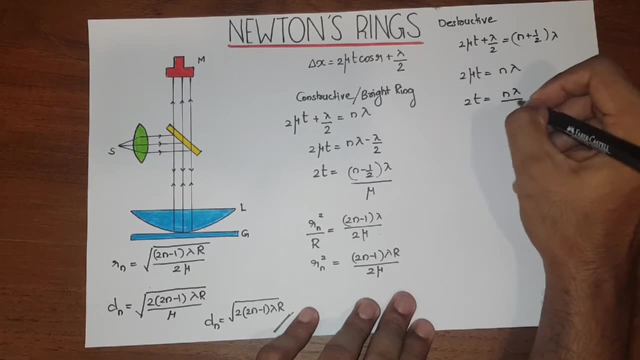 2 mu t can be arranged as n plus half lambda, minus lambda by 2 and writing it directly that is n lambda. Then 2 t can be written as n lambda by mu. So we know the value of 2 t. What is 2 t? 2 t is nothing. 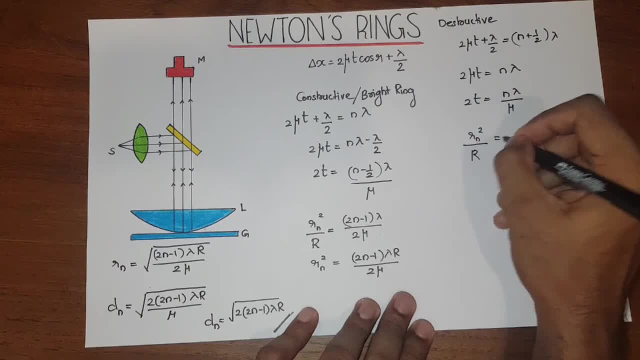 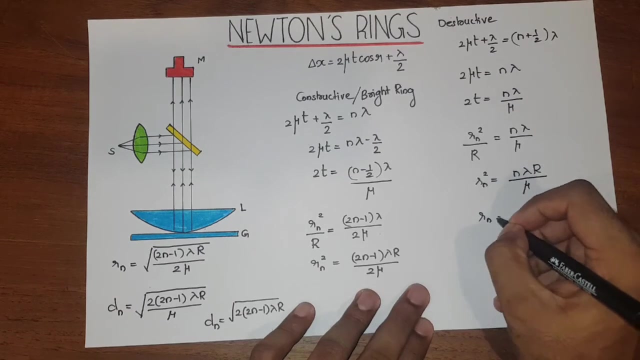 But r n square by r equals to n lambda by mu. Then the radius of the nth ring square is n lambda into the radius of curvature of the lens divided by refractive index of the medium. Then radius is the square root of this term, That is, n lambda r by mu From. 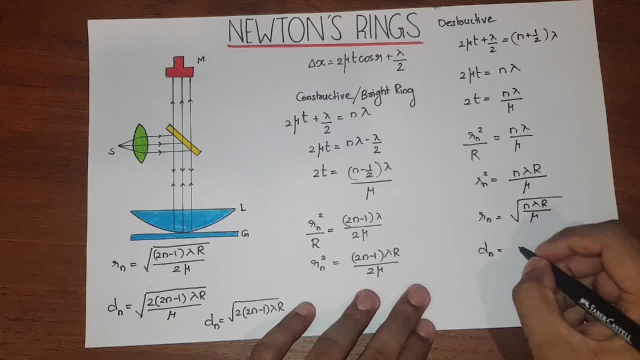 this you can write: the diameter Diameter of the nth ring is square root of this term, square root of 4n lambda r divided by mu. How does this 4 come into picture? Multiplying both sides by 2, this 2, when I took it inside the square root, it become 4.. Or if this mu value, 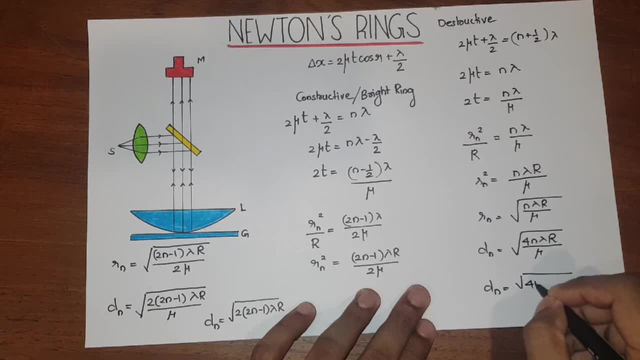 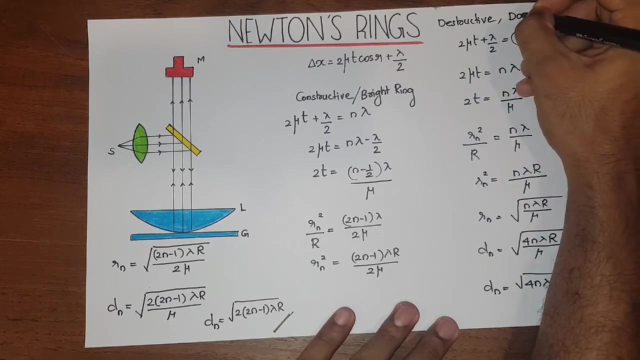 is 1, I can write it as: dn is equal to simply square root of 4n lambda r. So whichever ring that satisfies this condition, so whichever ring that has this diameter that satisfies this condition, it will be a ring where destructive interference is happening or it will be a 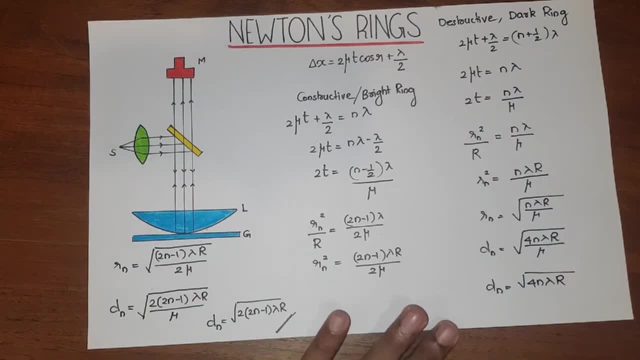 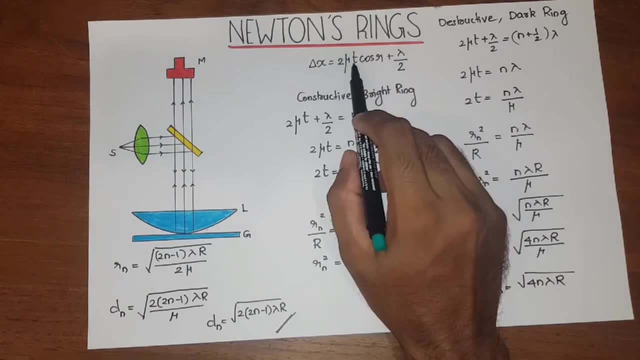 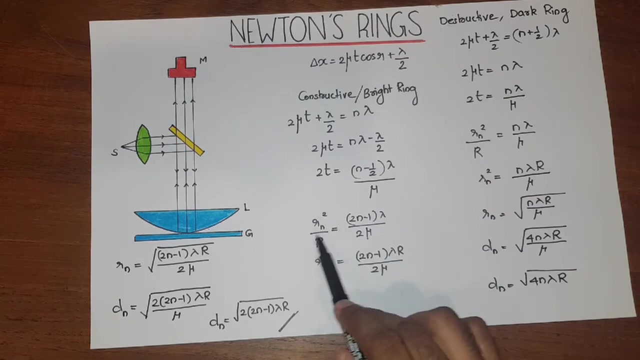 dark ring. So I already told you, if you look at this condition, this thickness will determine what kind of interference is happening at everywhere, Because this thickness is directly related to the radius of the nth ring. And why did we call it the ring? Because if we 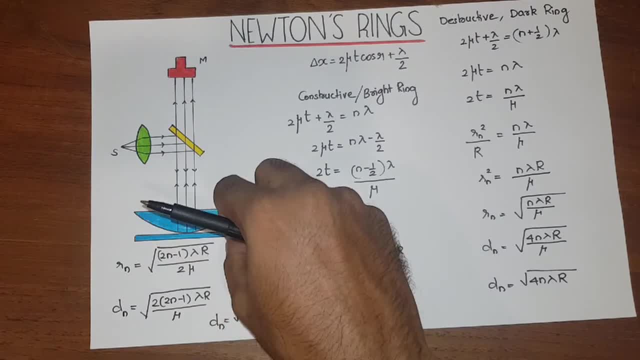 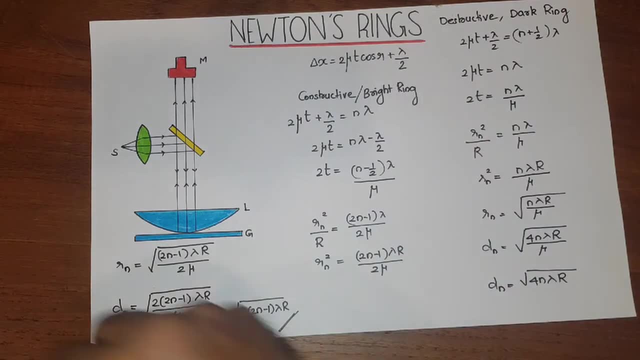 observe from, observe from the top, wherever the thickness has to be the same. if we collect all those points, or in other words I can say the locus of all the points where the thickness is the same will be a circle. So if you observe a fringe, that will be in the form of a circle. 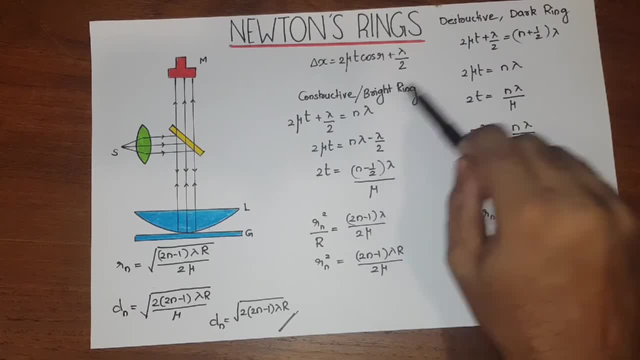 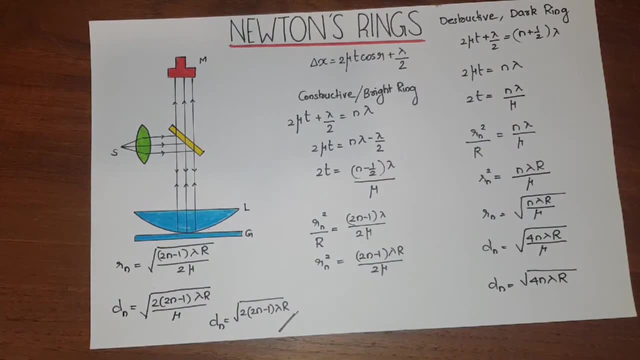 That is why I call the fringe as a ring. So instead of dark and bright fringe, I have to call it as dark and bright ring, which you can observe from the top. So this is the major conditions of Newton's ring. But now we have to discuss two major 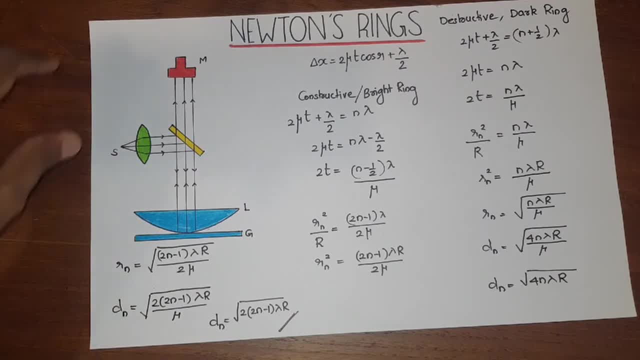 applications of Newton's ring, And one of them is to find out the wavelength of the light source which we are using. Simply by measuring the diameter, we will be able to know the wavelength of the light source that we are using. That is one application, And 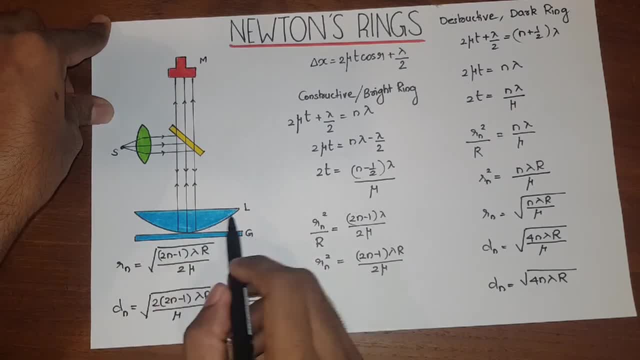 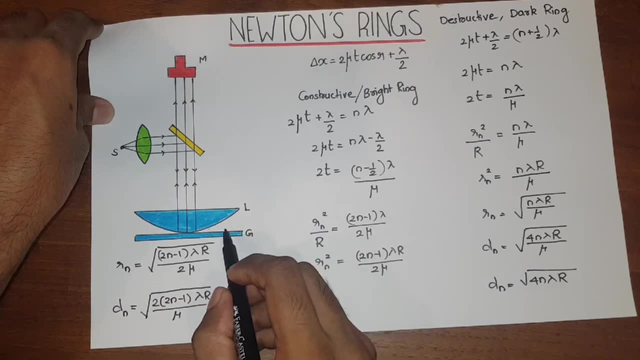 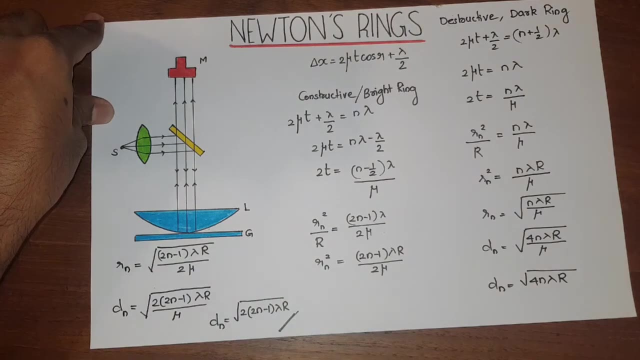 the other application is if, instead of air, if we are using some other material with some certain refractive index value, just by measuring the diameters we will be able to find out the refractive index of the material. So first of all, I am going to find out the wavelength. 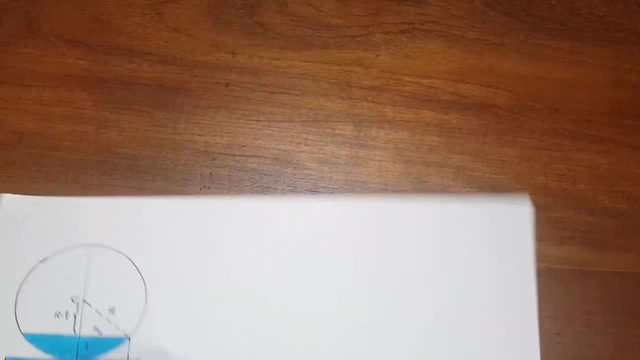 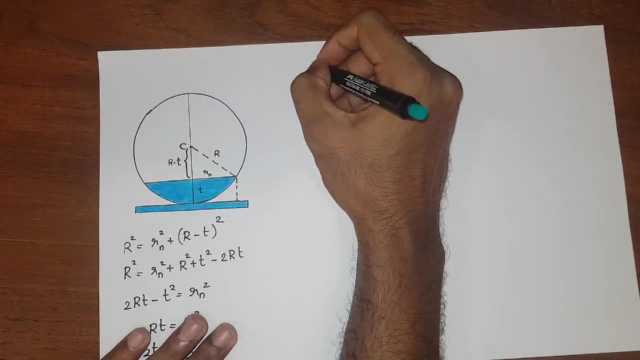 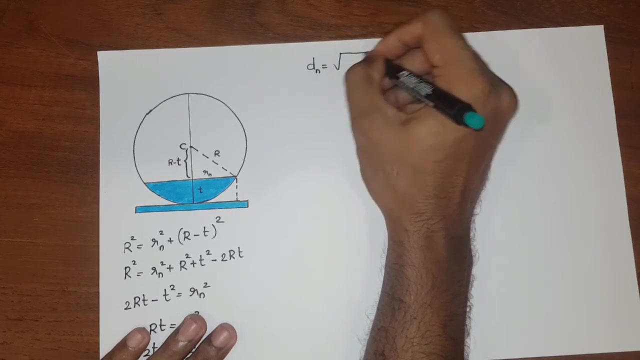 of the light source used with the help of Newton's ring. So for that, what we have to do is that I am taking a random ring and finding, measuring its diameter with the help of the microscope. We already know its formula, that is, square root of 4n lambda r. I am considering 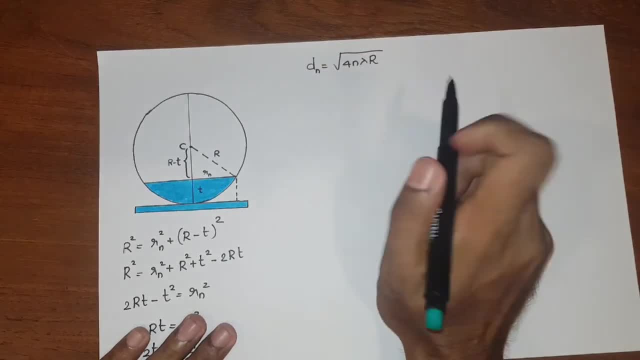 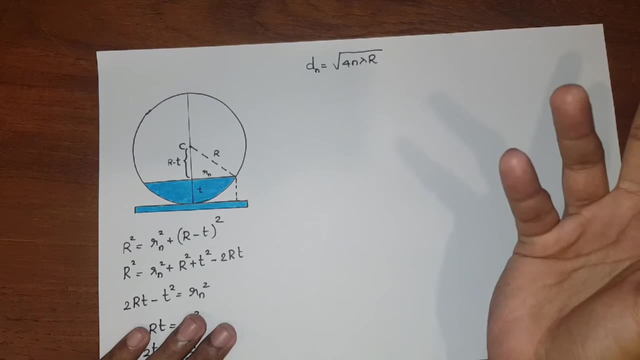 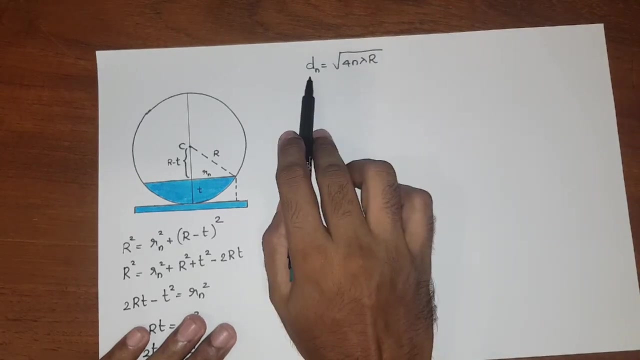 the case of the thin film, to be air. So the mu value is 1.. So I am neglecting the mu part. So I am just measuring the diameter of a random ring, some arbitrary ring. So we see the pattern. We choose some ring to be the nth ring And this is the diameter of the nth ring. So this: 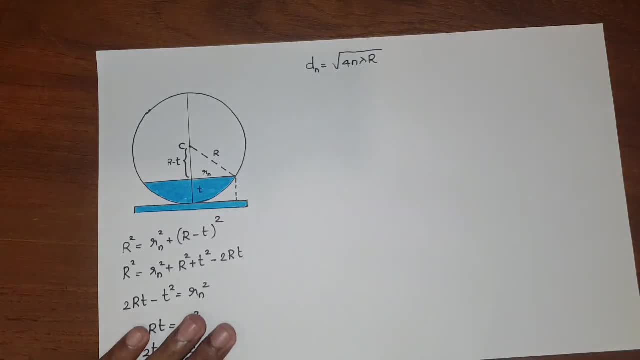 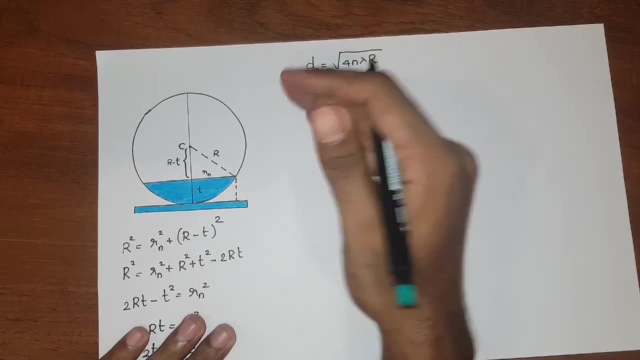 ring we will measure with the help of the microscope. So this is the diameter of the nth ring. So this distance we will measure with the help of the travelling microscope And after this I will measure the diameter of another ring, which is some k rings. after. 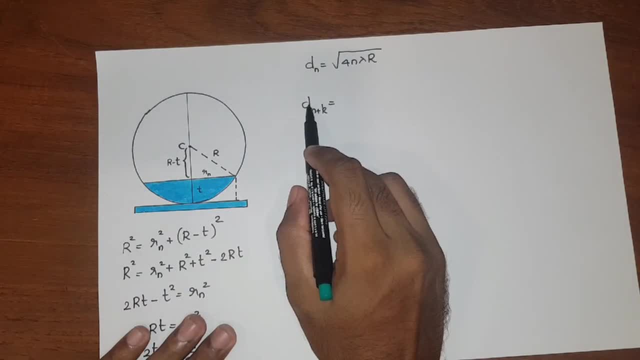 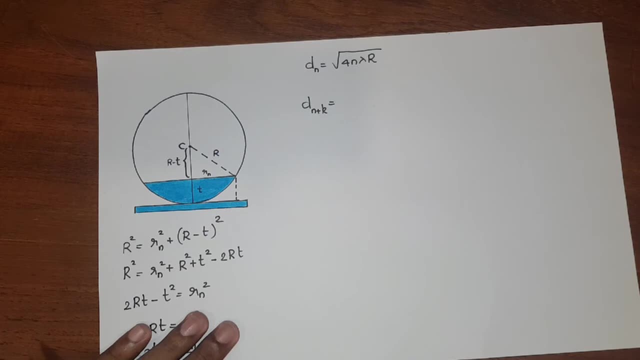 the nth ring. That is why I denoted the diameter of the second ring to be n plus kth rings diameter The n plus k. I hope it is clear. First we will choose the diameter. So this a ring from the pattern and that will be the nth ring. Now I will choose some other ring. 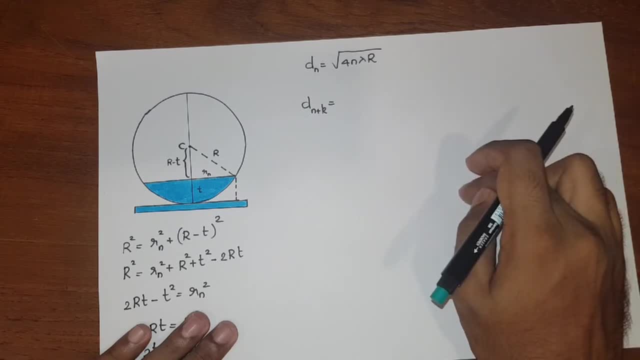 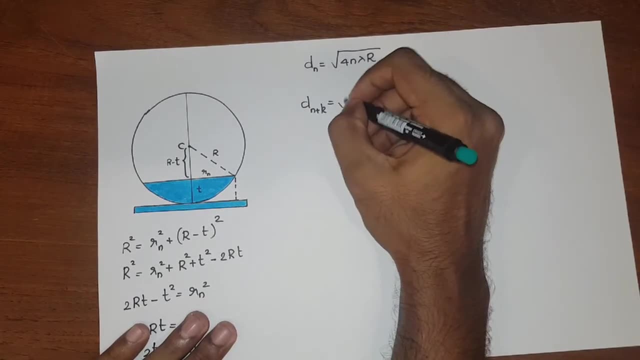 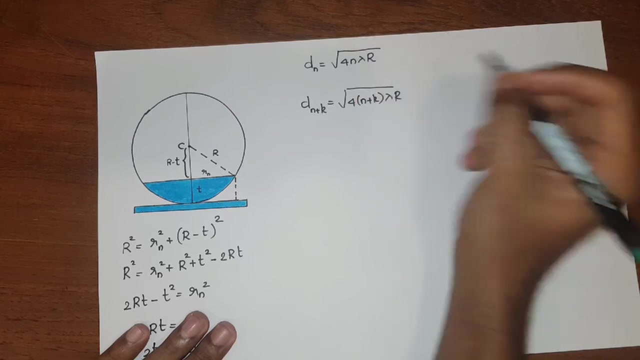 which is k rings. after the nth ring That will be a bigger ring, So I will measure its diameter and that will be the diameter d n plus k. And simply we can write in the formula like 4, n plus k into lambda r. instead of n I will put it as n plus k, So omitting the 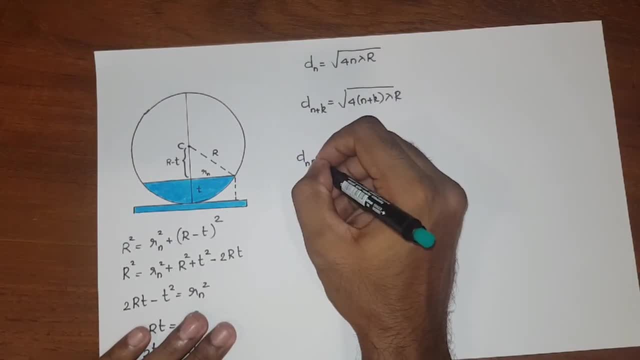 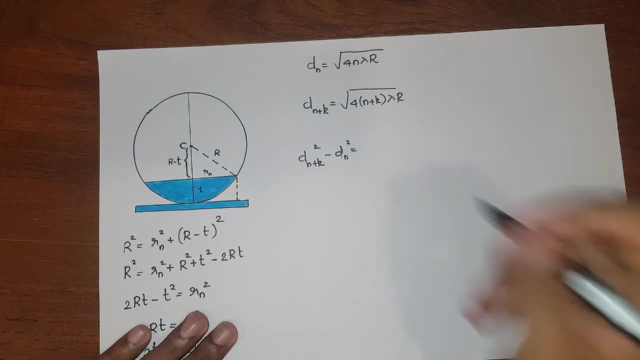 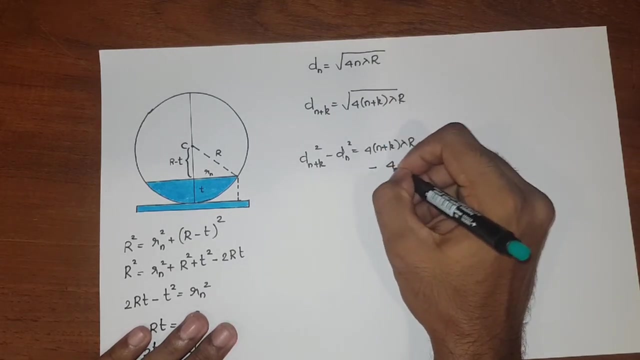 square root, or I am squaring these terms and then subtracting, what will we get? We will get 4 n plus k lambda r minus 4 n lambda r, And what? this will be 4 n lambda r and 4 n lambda r will cancel out and remaining it will be 4 n. 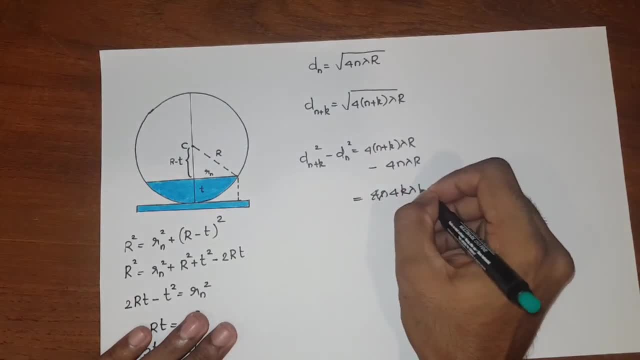 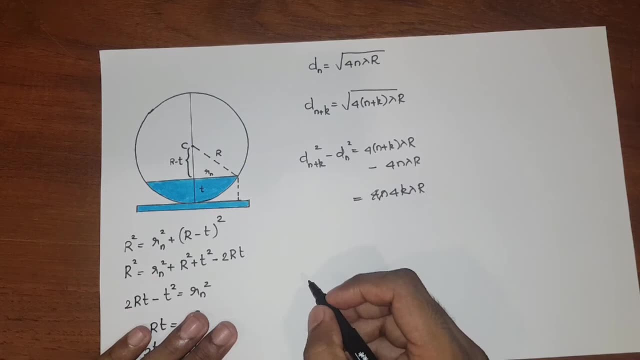 Sorry, it will be 4 k lambda r, The 4 n lambda r and 4 n lambda r will cancel. Remaining will be 4 k lambda r, And here we have the lambda which we require. So just rearrange that, So lambda will be equal to this term. that is d n plus k square minus d n square. 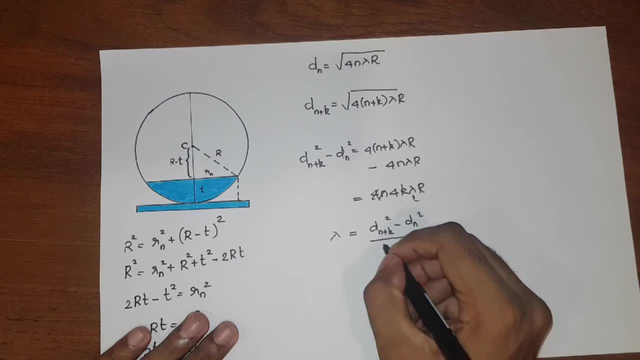 divided by. so retaining the lambda, I am bringing down 4 k n r. So we know the value of k and we know the value of k because from the arbitrary ring we are counting the number of rings, the kth ring. So we know the k, We know the. we should know the radius of curvature of. 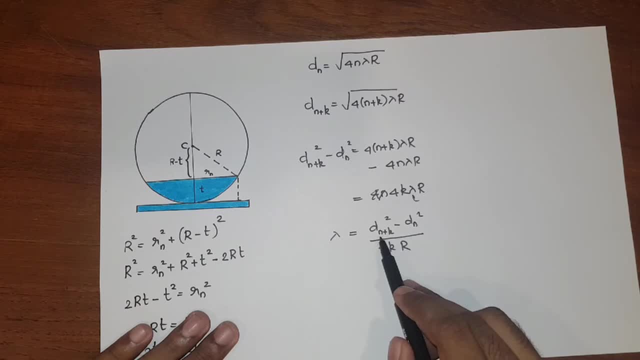 the lens which we are using. Then we just have to measure the diameter of the two rings: The first arbitrary ring, that is the nth ring, and from that we are measuring the kth ring and the diameter of that particular. So just by measuring the diameter of these two rings, 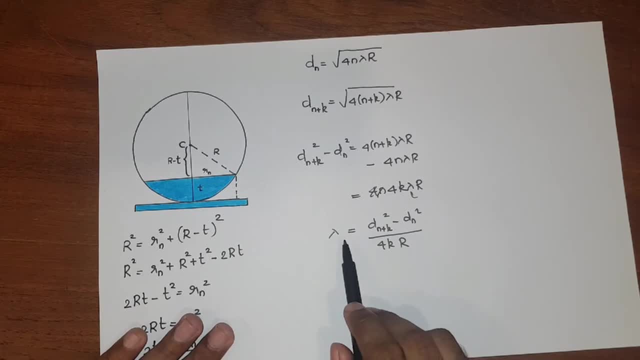 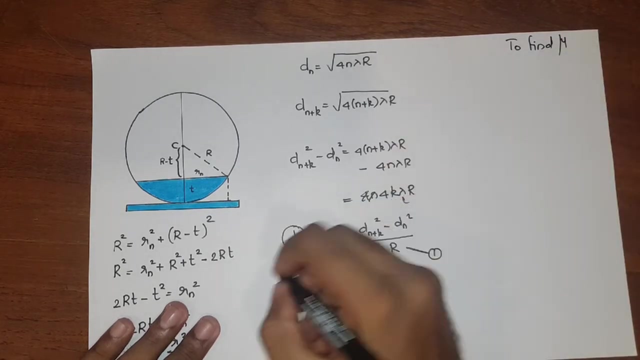 we have, we can find out the wavelength of the monochromatic source that we used to form this pattern. This is the first application of Nudel's law, And I am just marking these equations as 1.. Let it be there Now. the second application is to find mu, And this was to. 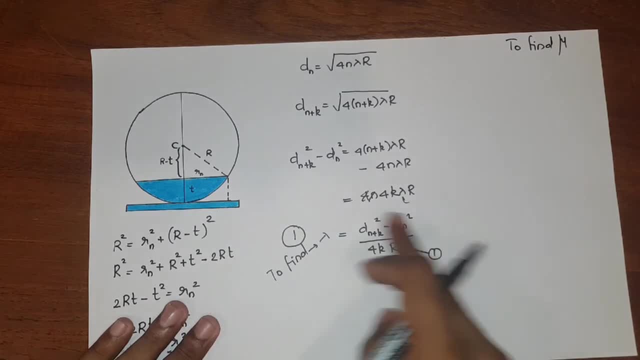 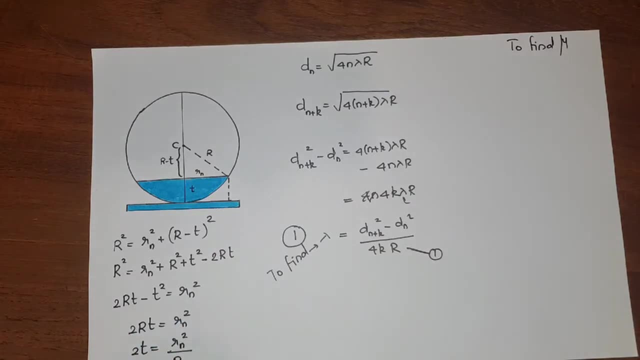 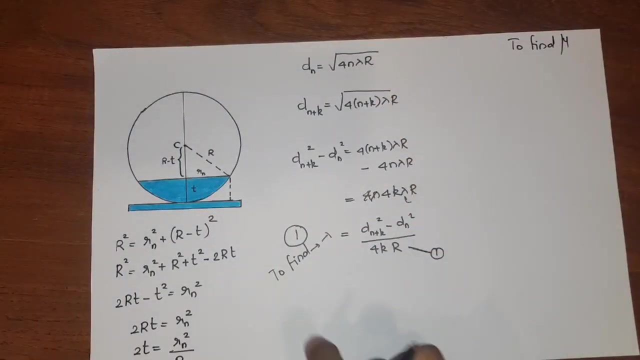 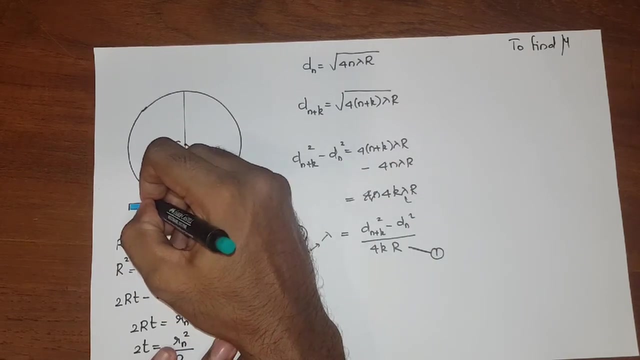 find lambda. This was done to find lambda. Now we are going to find the value of mu. So instead of using an air filler Right like here, first we were using an air film. that is how we did this experiment, and now, instead of air, I am choosing that there is some medium of refractive index mu over here. 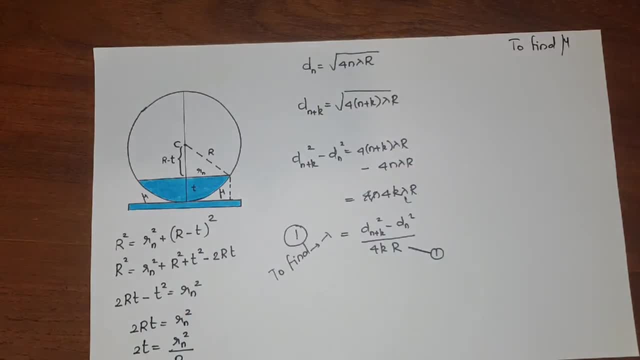 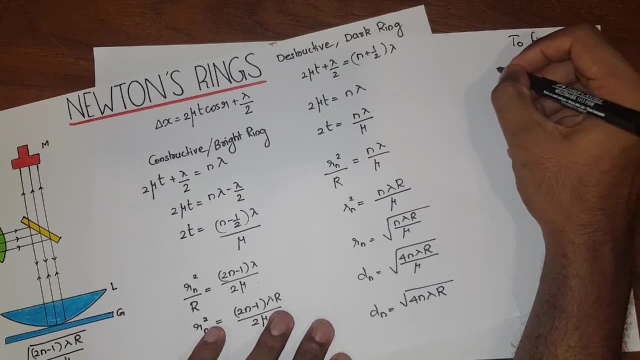 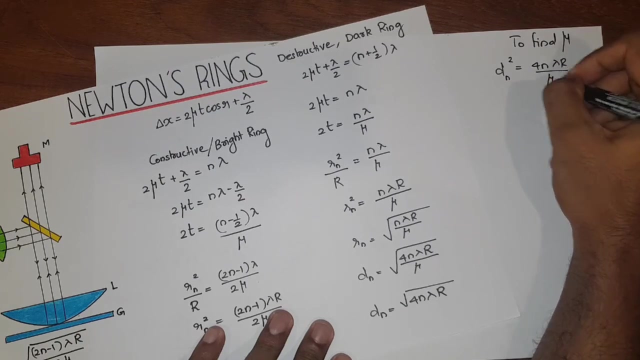 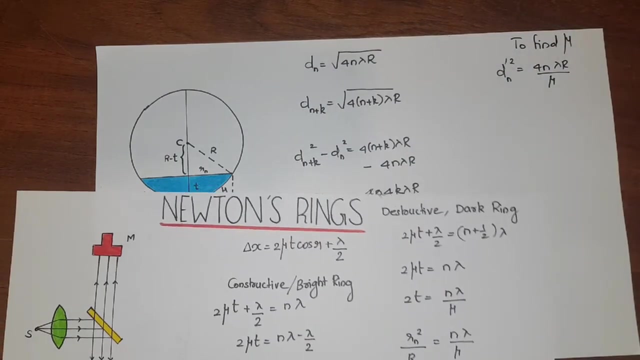 so what will be the formula for the diameters? you already know. so, before omitting the mu, what was the formula? dn was, so I am writing it as square dn, square equal to 4n lambda r by mu. so I cannot call this dn because dn. we already used it, so I called it as d dash. 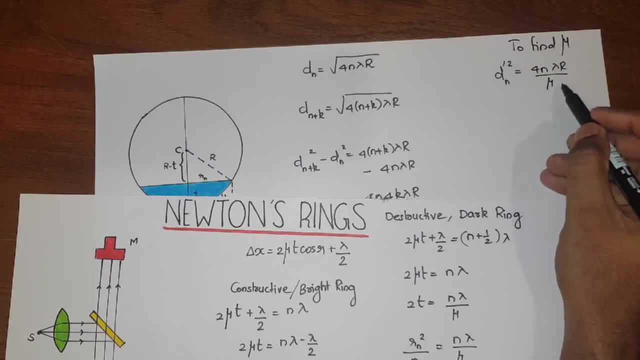 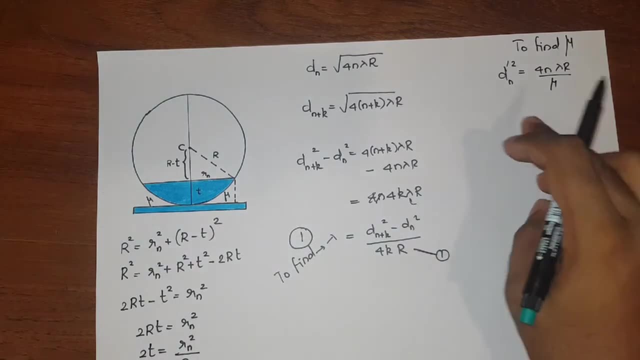 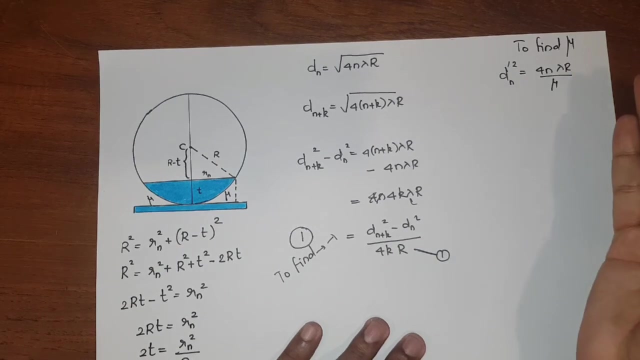 so d dash n square, that is 4n lambda r by mu when we are using a medium of refractive index, mu over here instead of air, and just like how we did, over here instead of the air, some adjacent rings. we will again measure the diameter of the kth ring. Remember we are doing. 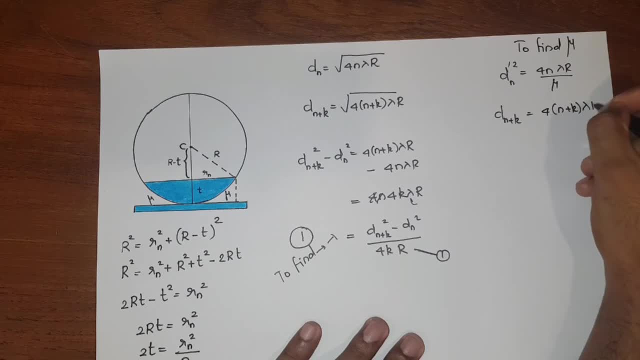 this thing with the help of some material that has a refractive index that is not equal to 1. If it was 1, then we will say that the case is that of air. Now, it is not air, we have a medium. 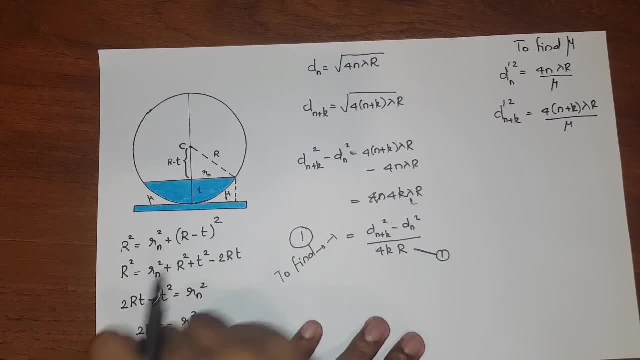 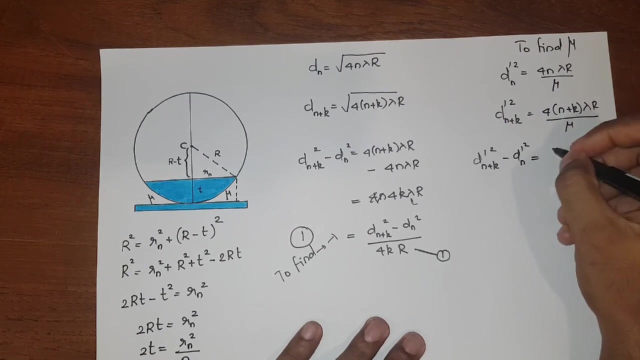 that has a refractive index, mu. alright, And again, I will measure these two distances and I can just subtract them: dn plus k square. that is, a dash minus dn. dash square will be the subtraction of these two terms. What will that be? 4n plus k lambda r by mu minus 4n lambda r by. 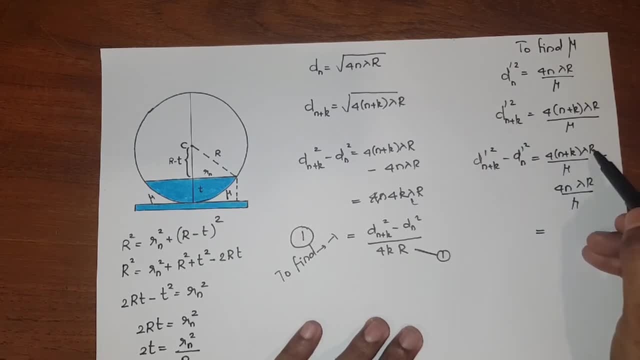 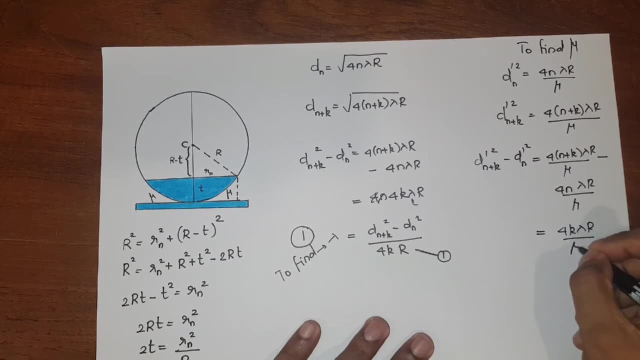 mu. This is nothing, but again what 4n lambda r by mu and 4n lambda r by mu will cancel out. Remaining is 4k lambda r by mu. that is dn plus k dash square, minus dn dash square. Can we do something with? 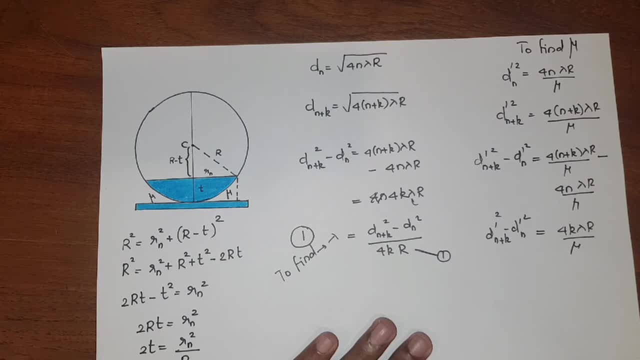 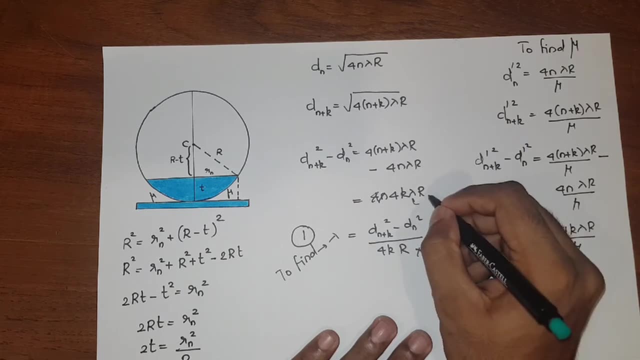 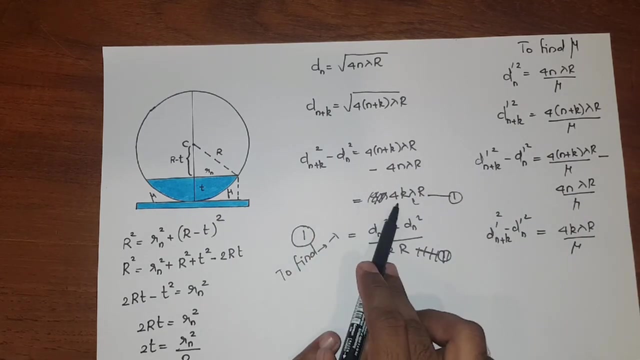 this. So now I am choosing this equation. Sorry, I call this equation as 1, sorry, I am going to call this equation as 1.. That is dn plus k square minus dn square is equal to- sorry, 4k lambda r. Now I am dividing the first equation with the second one. What will I get? 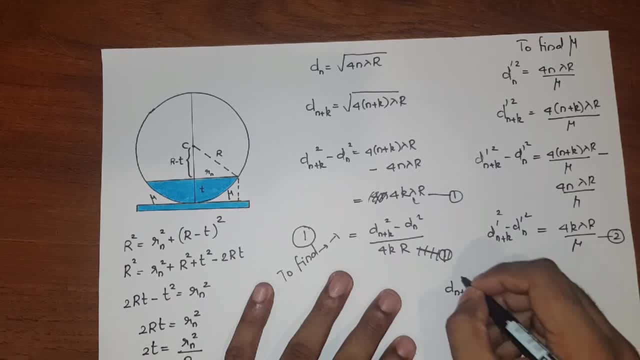 Alright, So dn plus k square minus dn square, that is the left-hand side. Right-hand side is dn plus k dash square minus dn dash square, equal to right-hand side of this term. 4k lambda r divided by 4k lambda r by mu. These things will be cancelled out and this will be mu.